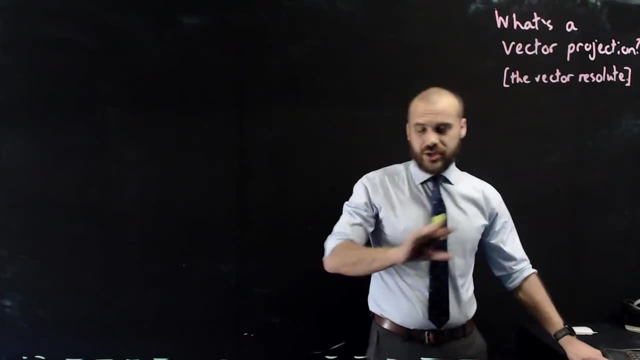 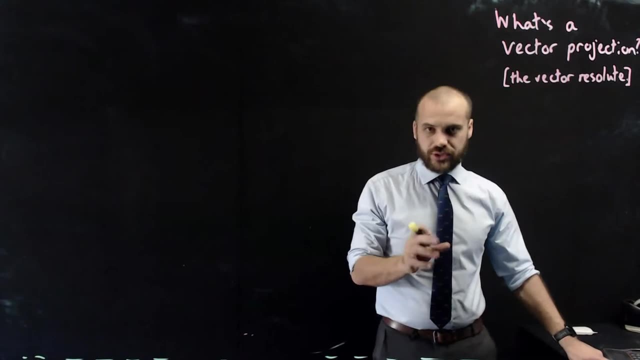 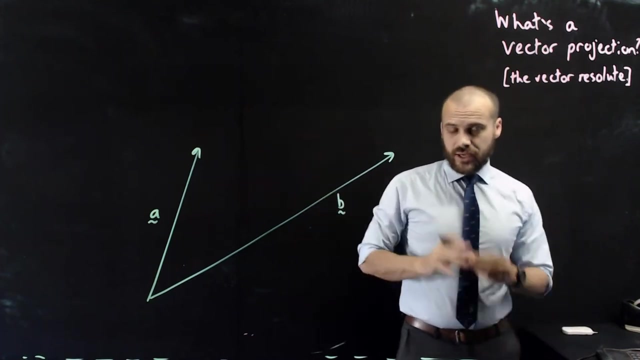 Alright, so this is a video just to explain what a vector projection is. No calculations in this one, just explain a fairly complicated topic that people really sort of struggle with at times. Alright, so let's jump into it. We need a picture. So here are my two vectors, A and B. Now I'm going to do a vector projection. That means I'm going to project one vector onto another vector, and for that I'm going to need a torch. 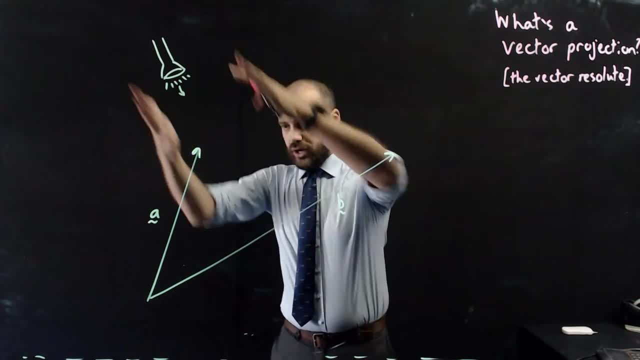 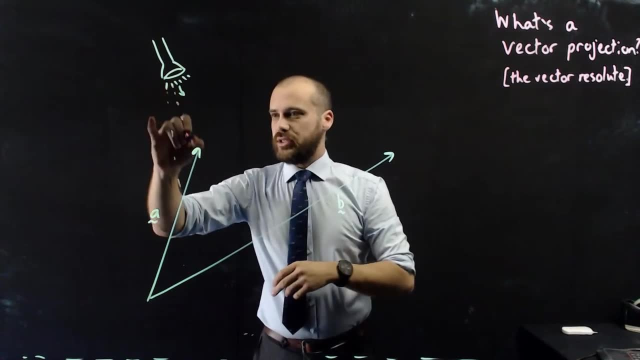 Now there's my torch, and my torch is going to cast light in this direction. Now it's going to. the light's going to go that way. and hit vector A, the light's going to go that way. and hit vector A, the light's going to go that way. 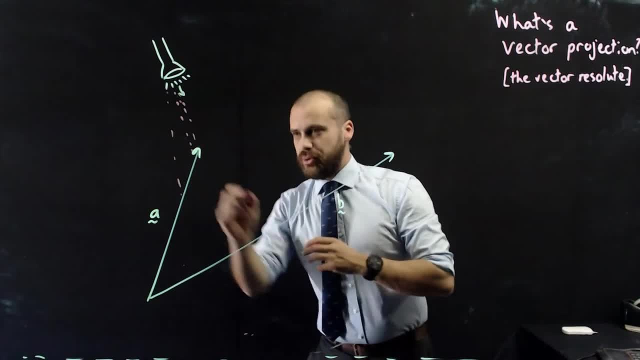 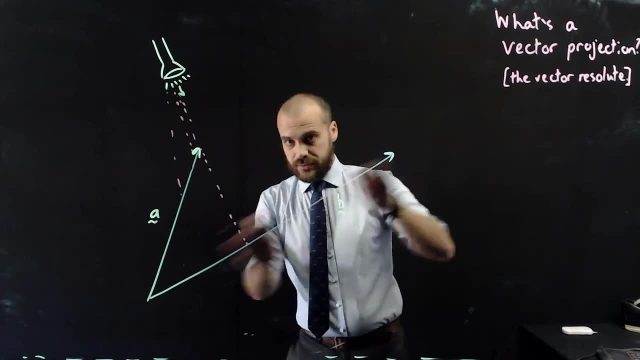 The light's going to go that way and just pass by vector A. Now that torch is making a right angle with vector B, so it's perpendicular to vector B, which means that we get this nice little right angle. Here's my torch. 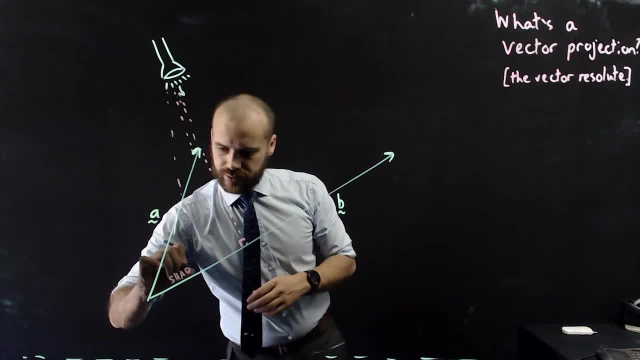 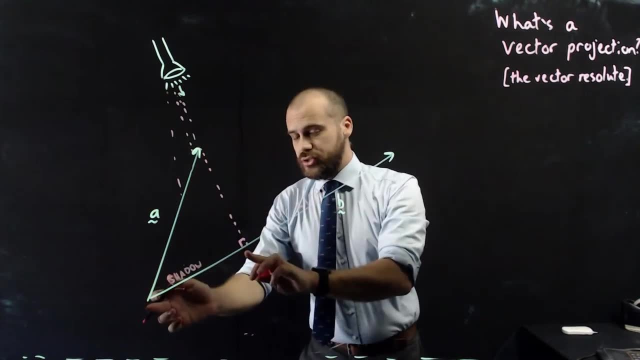 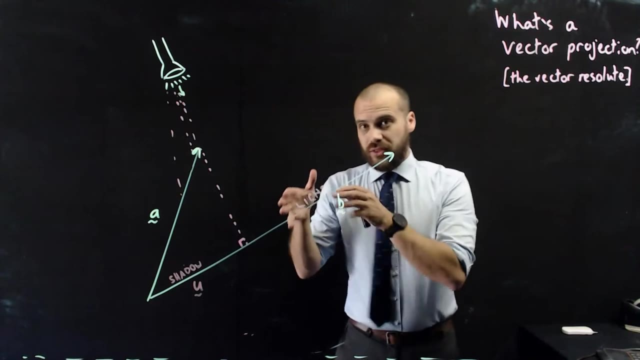 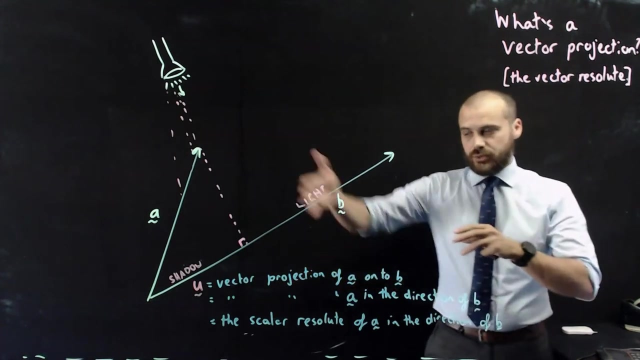 Here This is shadow And this is light. Now the vector projection of A onto B is the shadow. So this is vector U And I can call vector U the vector projection of A onto B, The vector projection of A onto B. So we're projecting A onto B. We can also say it's the vector projection of A in the direction. 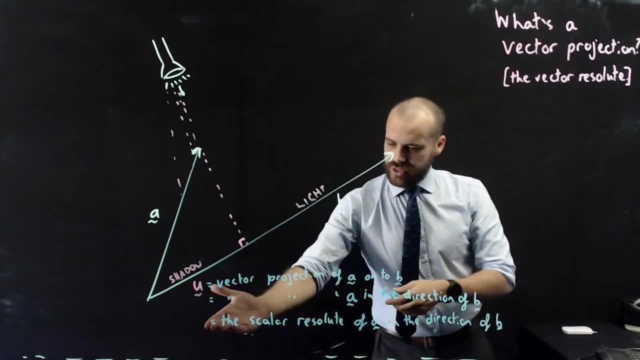 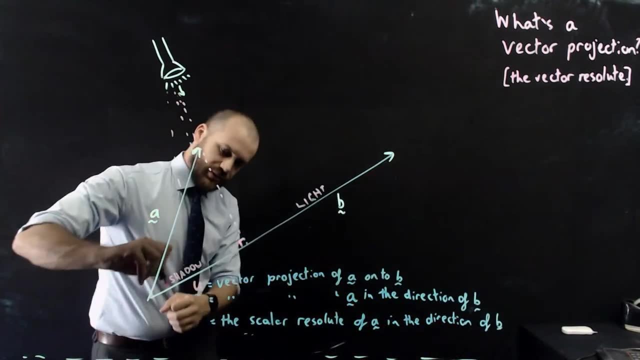 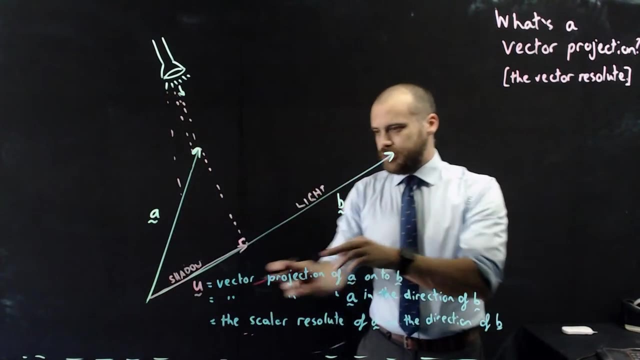 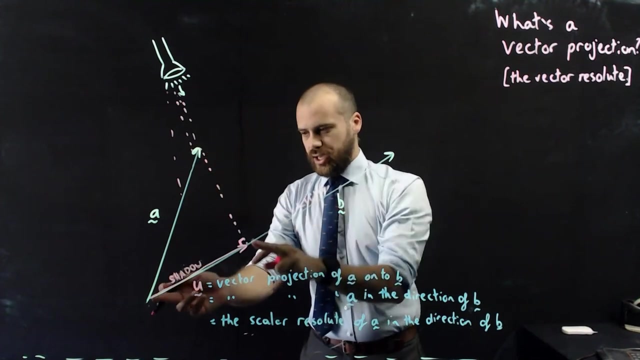 of B. We can also say that it is the scalar resolution resolute of A in the direction of B. So make no mistake, it is a vector, That is vector U. You can see a couple of things. In this particular instance- or I'm going to say in all instances- it's going to be smaller than vector A. here the shadow. 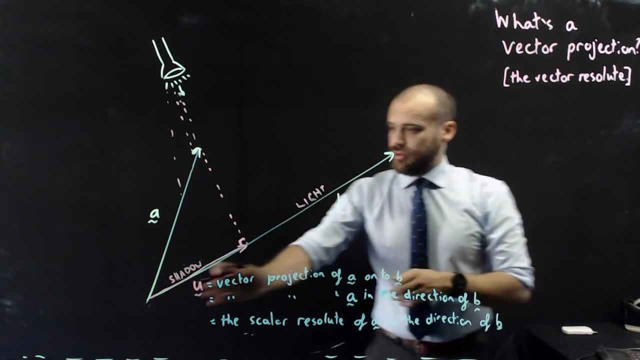 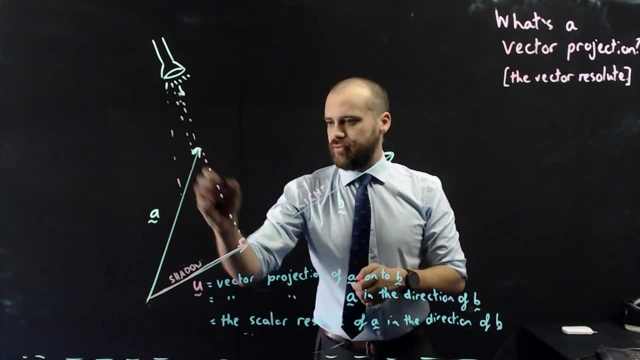 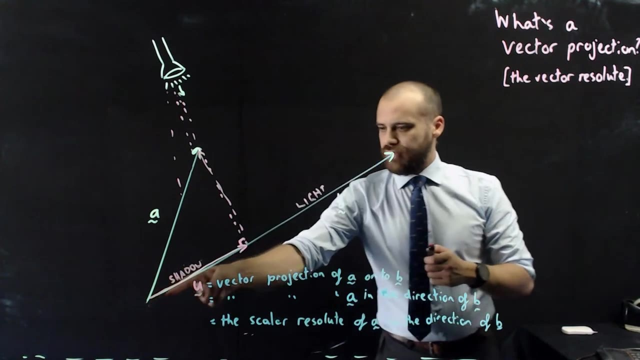 Now we can say that there is this vector here, U, which is the vector projection of A onto B, And then there's also this other vector here which doesn't have a fancy name. But if we were to add the vector projection of A onto B and then this other vector on here, we would actually get vector A.